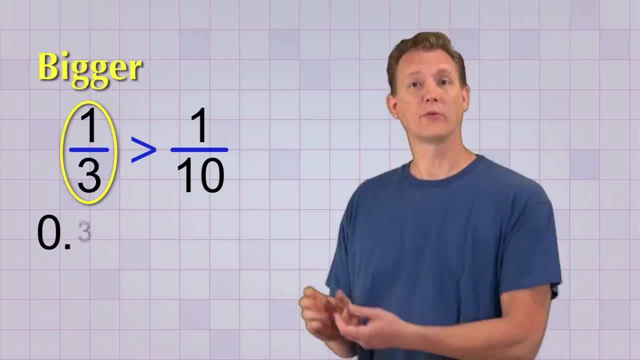 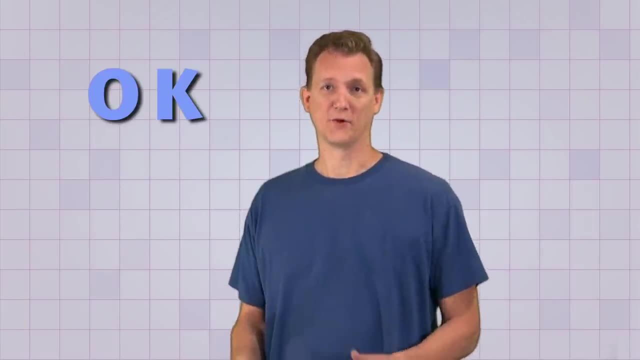 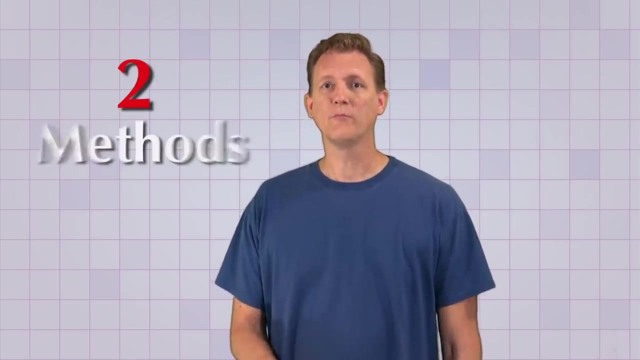 decimal value. what you get when you divide is 0.33333,, but the value of 1 over 10 is only 0.1.. Okay, so comparing fractions isn't quite as easy as comparing regular numbers, but that doesn't mean it's going to be that hard. We're going to learn two methods for comparing. 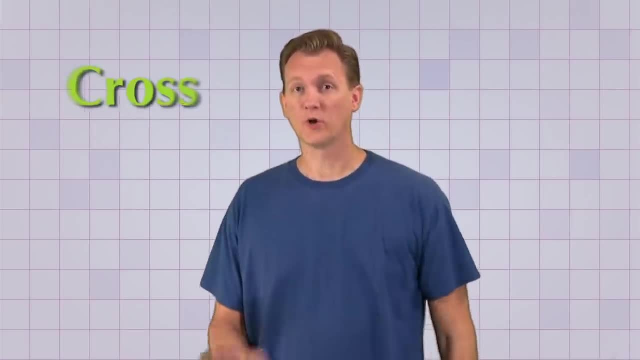 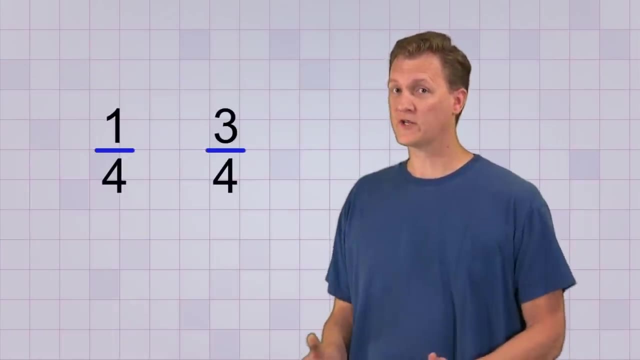 fractions. that make it very easy. The first method is called cross-multiplying and it takes advantage of the fact that it's easy to compare fractions with the same bottom numbers. If two fractions have the same bottom numbers, then we can just compare the top numbers. That's because 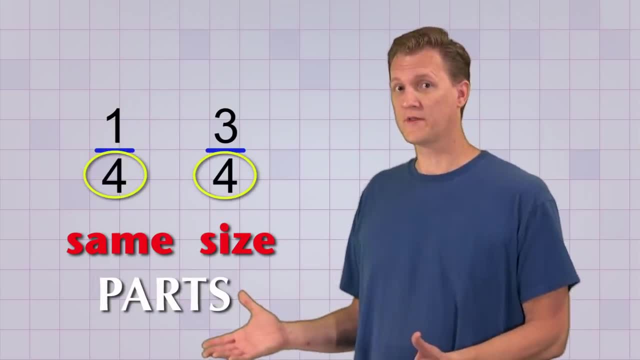 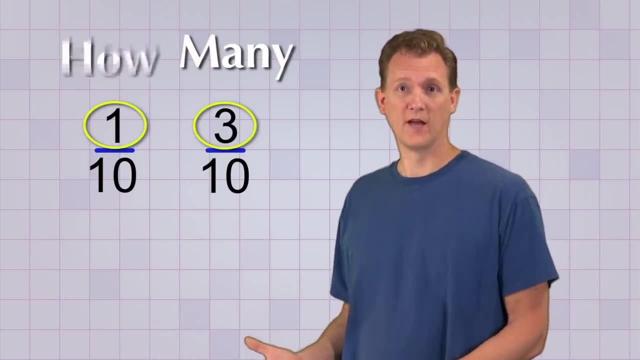 we're comparing the same size parts, We're comparing fourths to fourths, eighths to eighths, tenths to tenths and so on, And the top number just tells us how many of those parts we have. so it's easy to see that 5 eighths is more than 3 eighths. 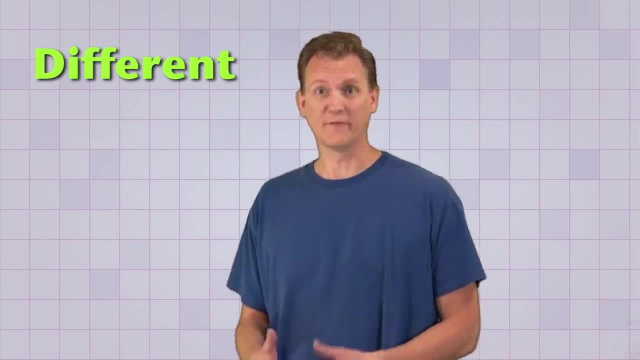 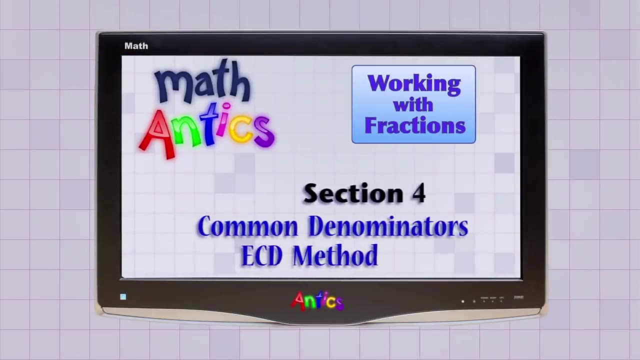 Many times you'll have to compare fractions that have different bottom numbers or different size parts. Fortunately, there's a trick we can do to make the comparison easy. In the Math Antics videos about common denominators we learn a simple method for. 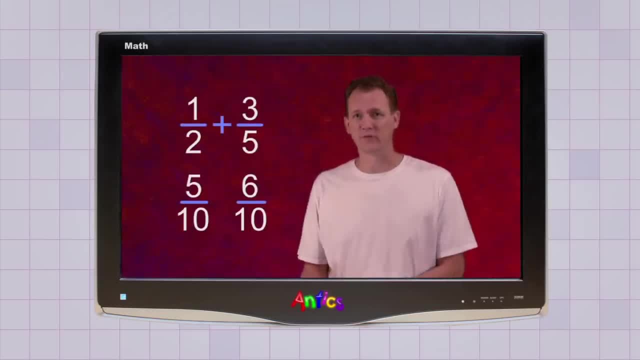 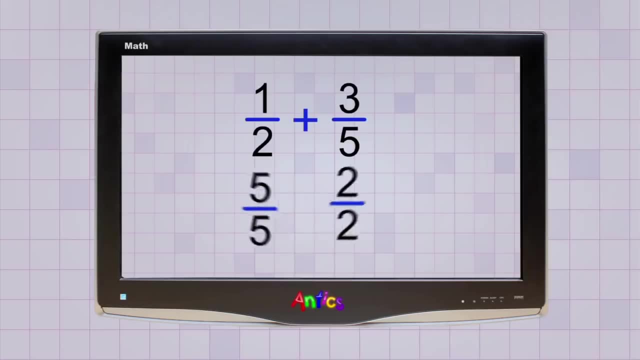 changing unlike fractions with different bottom numbers into like fractions with the same bottom number. Basically, it shows how you can multiply two unlike fractions by whole fractions made from the different bottom numbers, so you end up with the same bottom number. This will give you two new. 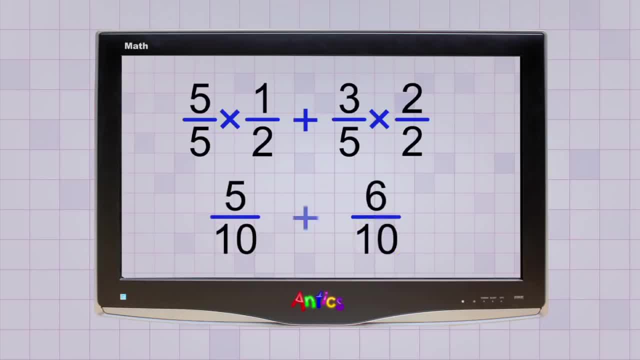 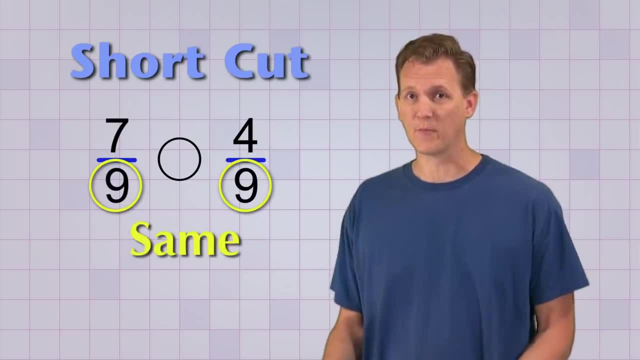 equivalent fractions that you can easily add, subtract or compare. But there's a shortcut for comparing fractions. As long as we know that the bottom numbers of our fractions are the same, we don't really need to know what that number is. We just need to know. 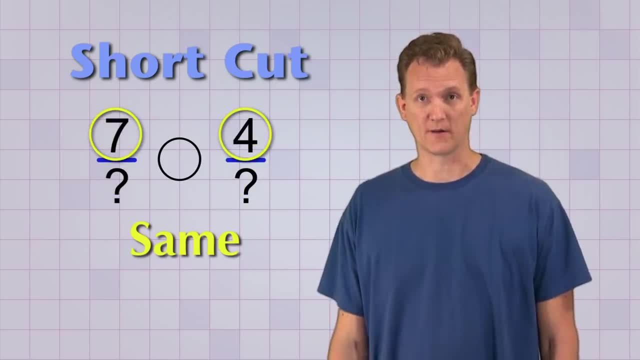 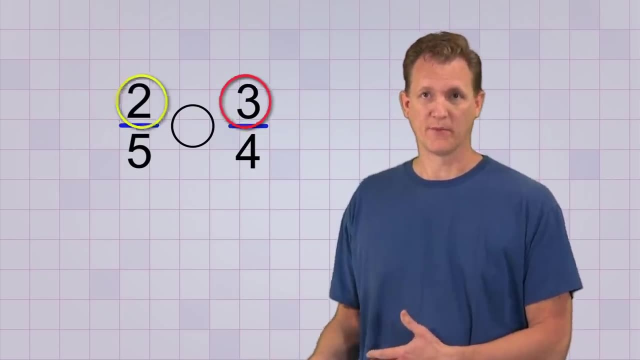 what the top numbers will be, since those are the ones that we'll actually compare. So instead of multiplying each fraction by a whole fraction, we can just multiply the top number of each fraction by the bottom number of the other fraction. This is called cross-multiplying. 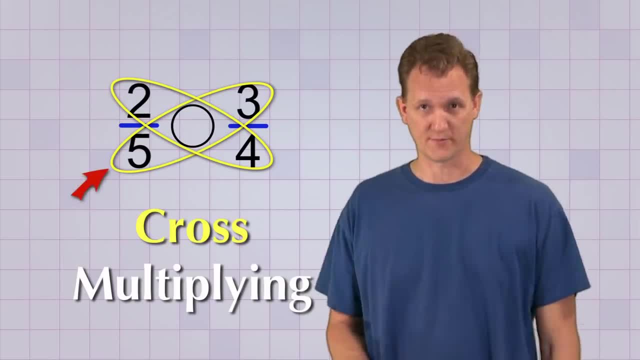 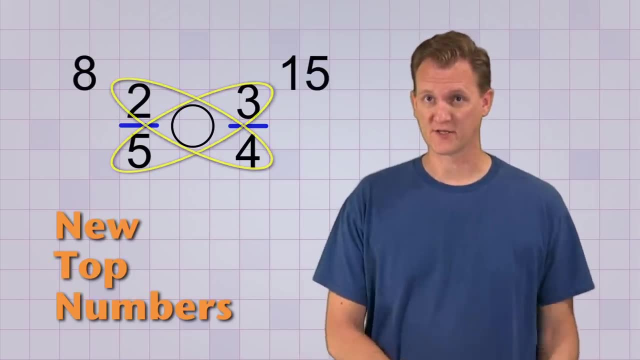 because if you draw a diagram of what you're multiplying, it forms a criss-cross pattern. After you cross multiply, you'll have two numbers- that would be the new top numbers if you had made like fractions, and those numbers will show you which fraction is greater. 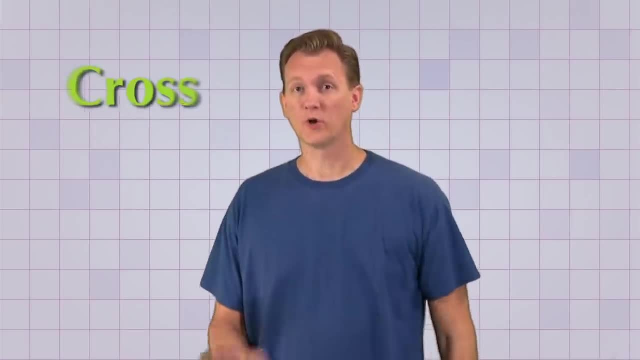 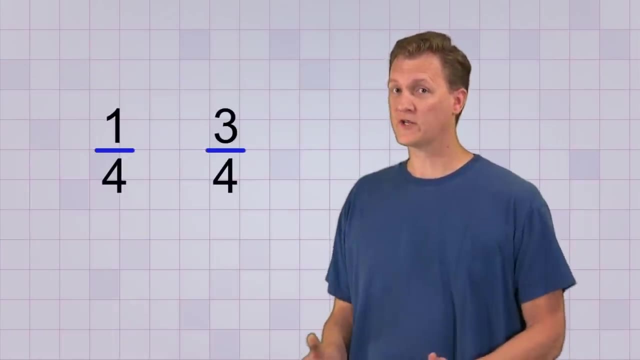 fractions. that make it very easy. The first method is called cross-multiplying and it takes advantage of the fact that it's easy to compare fractions with the same bottom numbers. If two fractions have the same bottom numbers, then we can just compare the top numbers. That's because 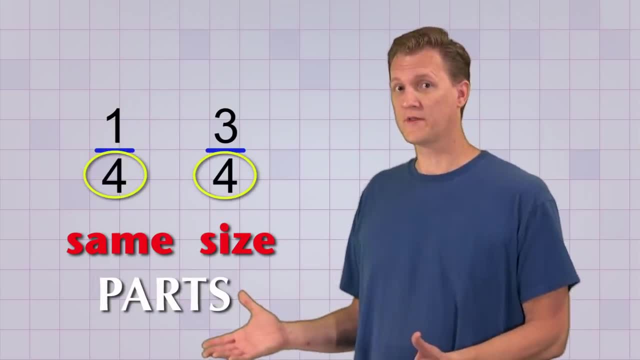 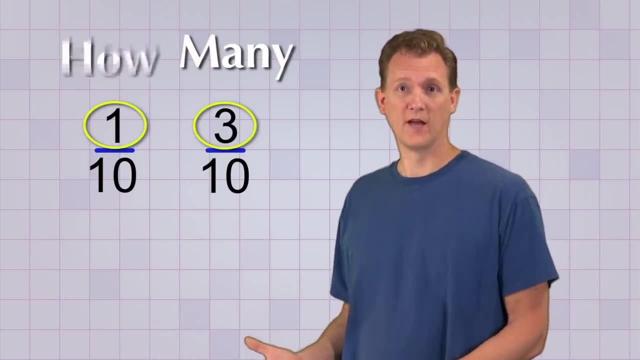 we're comparing the same size parts, We're comparing fourths to fourths, eighths to eighths, tenths to tenths and so on, And the top number just tells us how many of those parts we have. so it's easy to see that 5 eighths is more than 3 eighths. 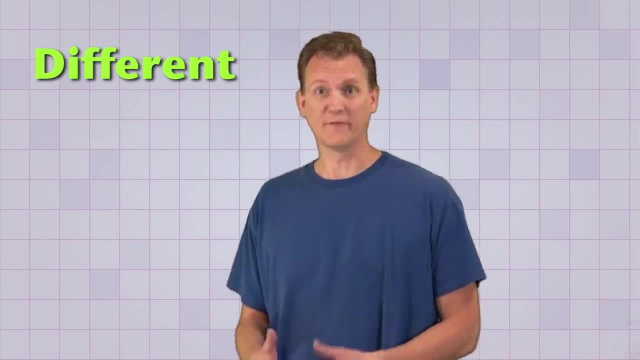 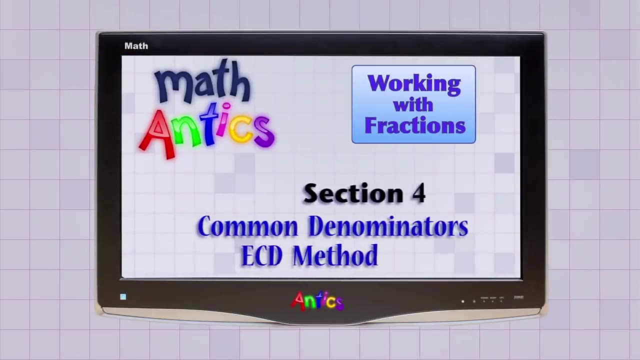 Many times you'll have to compare fractions that have different bottom numbers or different size parts. Fortunately, there's a trick we can do to make the comparison easy. In the Math Antics videos about common denominators we learn a simple method for. 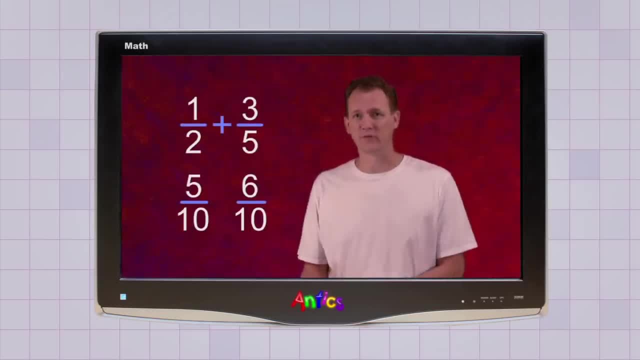 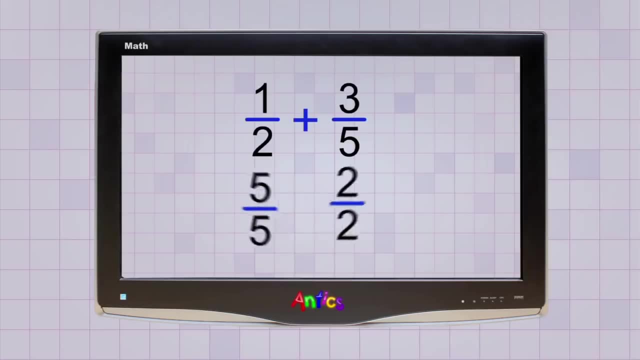 changing unlike fractions with different bottom numbers into like fractions with the same bottom number. Basically, it shows how you can multiply two unlike fractions by whole fractions made from the different bottom numbers, so you end up with the same bottom number. This will give you two new. 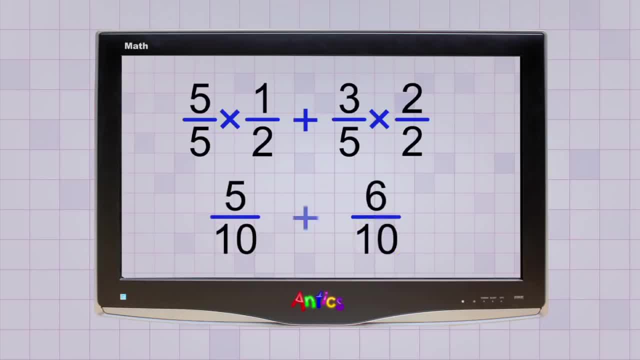 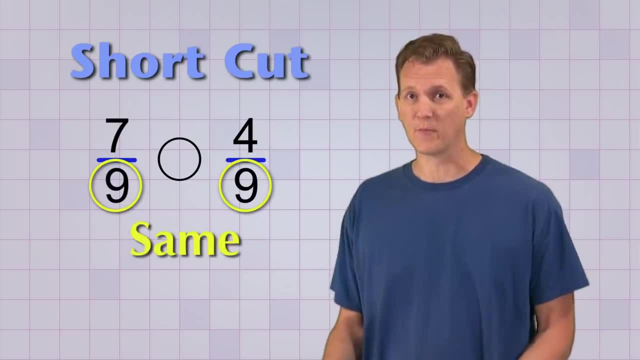 equivalent fractions that you can easily add, subtract or compare. But there's a shortcut for comparing fractions. As long as we know that the bottom numbers of our fractions are the same, we don't really need to know what that number is. We just need to know. 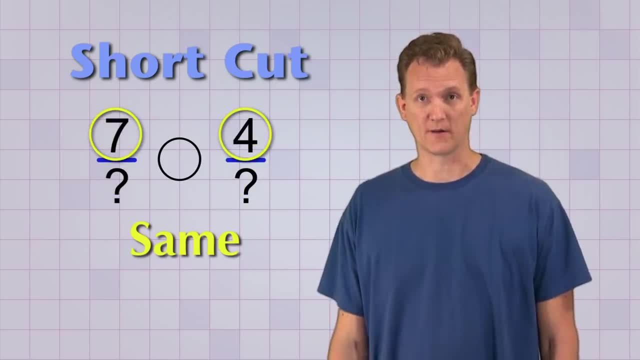 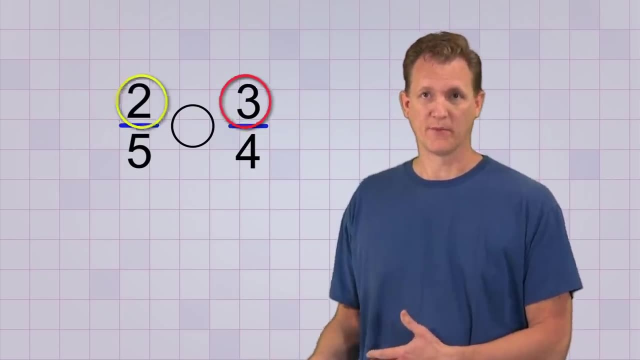 what the top numbers will be, since those are the ones that we'll actually compare. So instead of multiplying each fraction by a whole fraction, we can just multiply the top number of each fraction by the bottom number of the other fraction. This is called cross-multiplying. 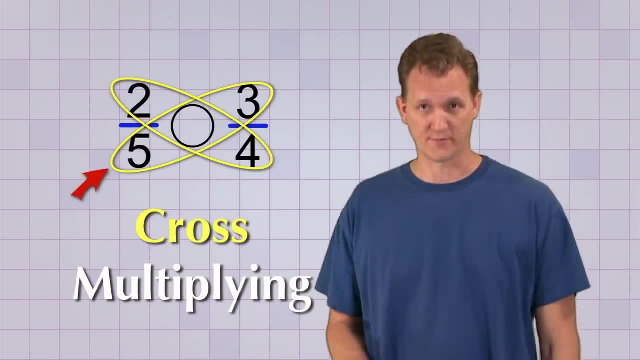 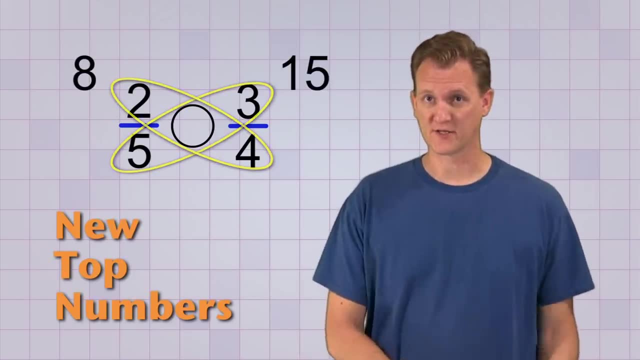 because if you draw a diagram of what you're multiplying, it forms a criss-cross pattern. After you cross-multiply you'll have two numbers- that would be the new top numbers if you had made like fractions, and those numbers will show you which fraction is greater. 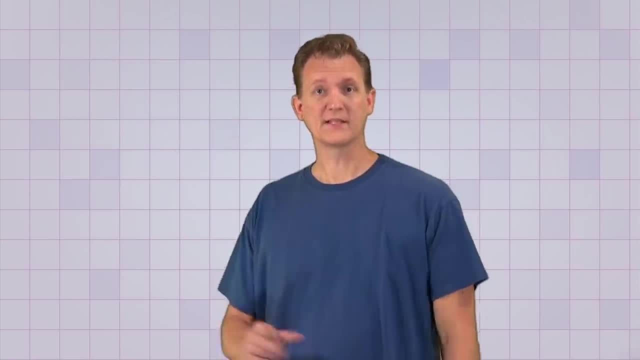 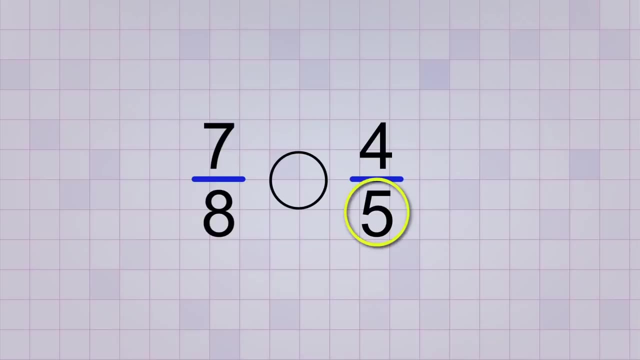 Let's try this cross-multiplying method on an example or two. Let's compare the fractions 7 over 8 and 4 over 5.. We start by multiplying the second fraction's bottom number, 5,, by the first fraction's top number, 7, and that gives us 35. 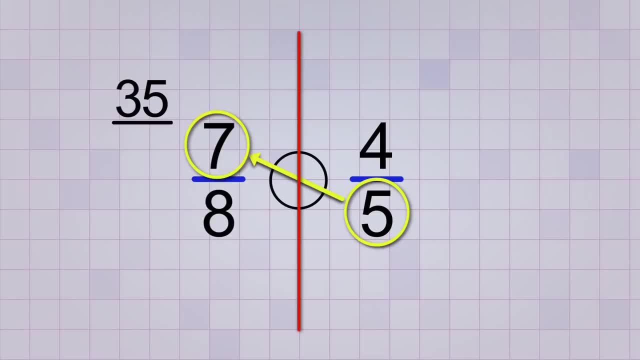 top number on this side. You'll always keep the answer on the side of the top number that you multiplied. Now for the other side, The bottom number 8, times the top number 4, gives us 32 for its new top number. 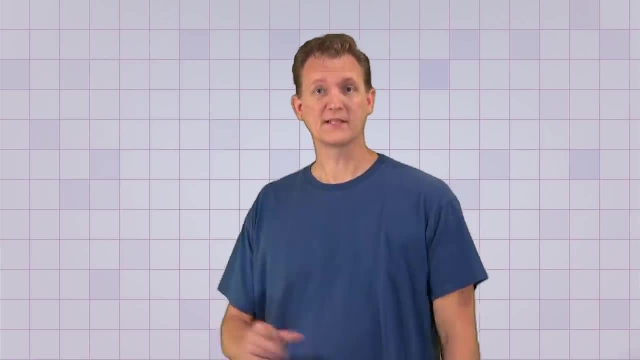 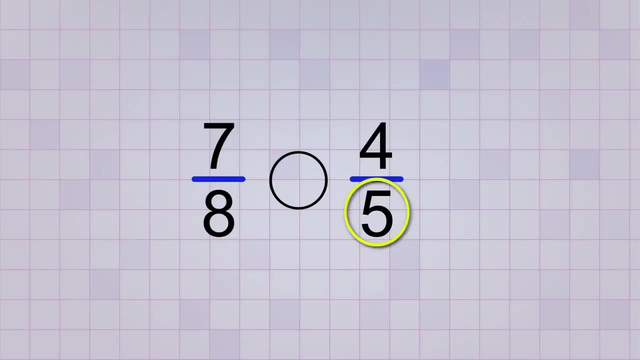 Let's try this cross-multiplying method on an example or two. Let's compare the fractions 7 over 8 and 4 over 5.. We start by multiplying the second fraction's bottom number, 5,, by the first fraction's top number, 7, and that gives us 35. 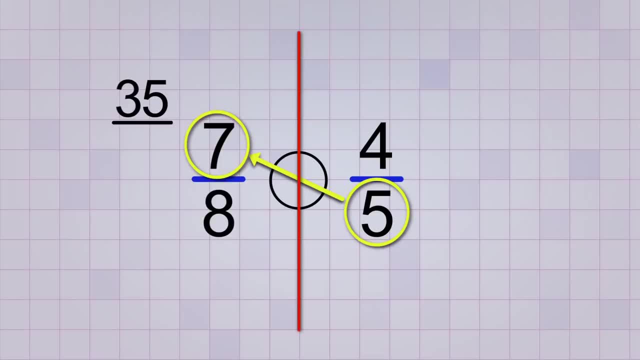 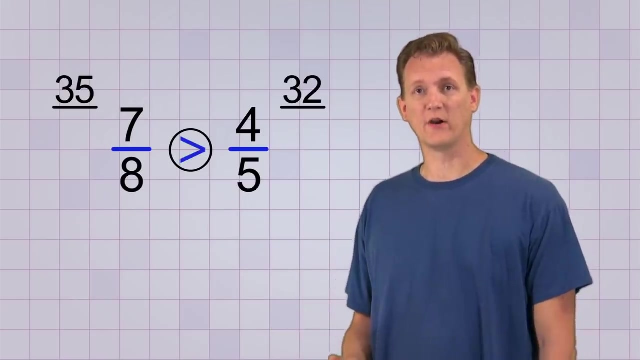 top number on this side. You'll always keep the answer on the side of the top number that you multiplied. Now for the other side, The bottom number 8 times the top number 4 gives us 32 for its new top number. Aha, Now it's easy to see that the fraction 7 over 8 is greater than the fraction 4 over. 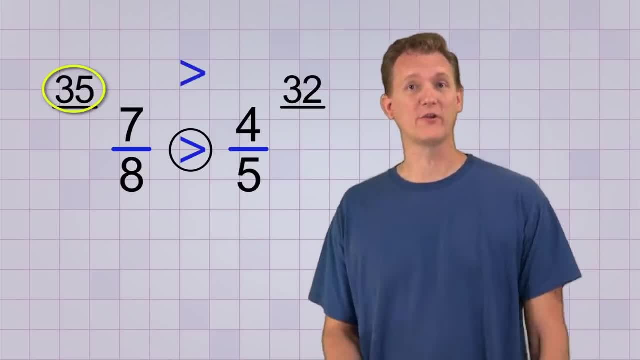 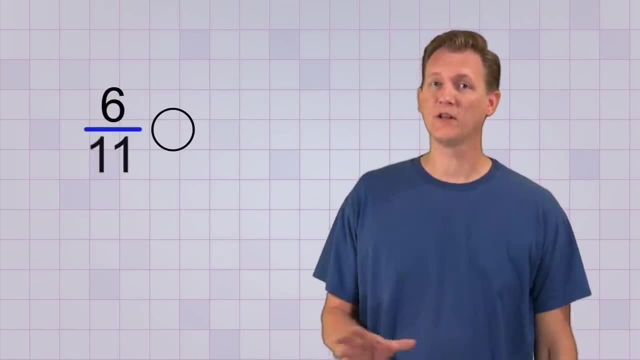 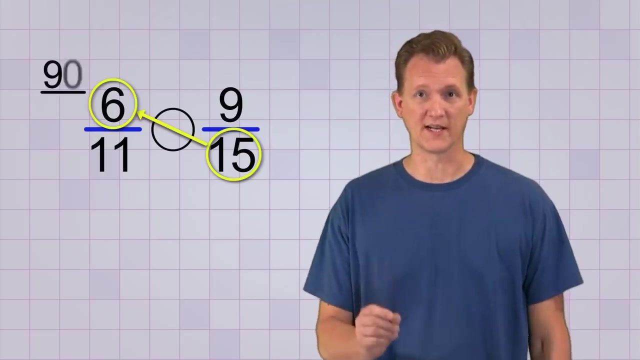 5 because its new top number, 35, is greater than the other new top number 32.. Let's do one more comparison by cross-multiplying. Let's compare 6 over 11 to 9 over 15.. First we'll multiply 15 by 6 to get the new top number of the first side, which is 90.. 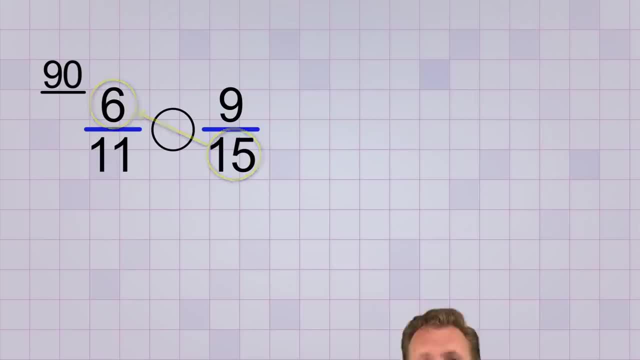 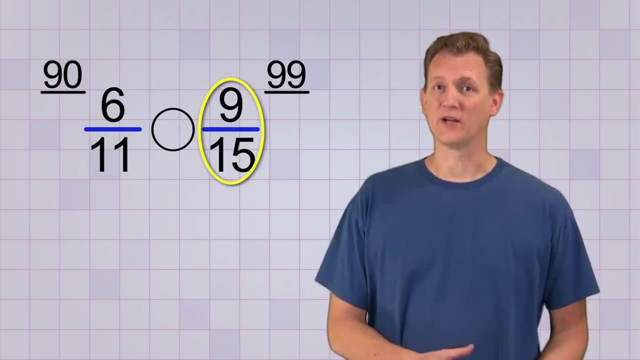 You can always use a calculator to do the multiplications if you need to. Next, we multiply 11 by 9 to get the second new top number, which is 99.. So that tells us that the second fraction- 9 over 15, is greater than the first fraction. 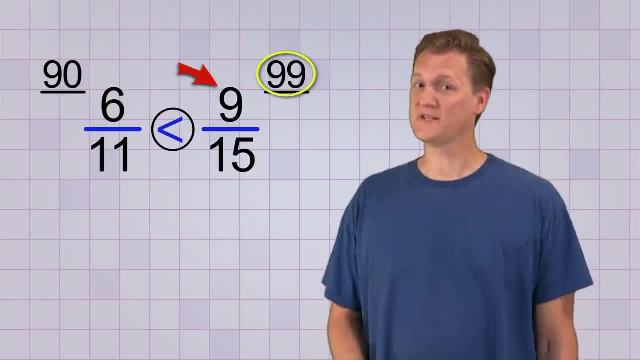 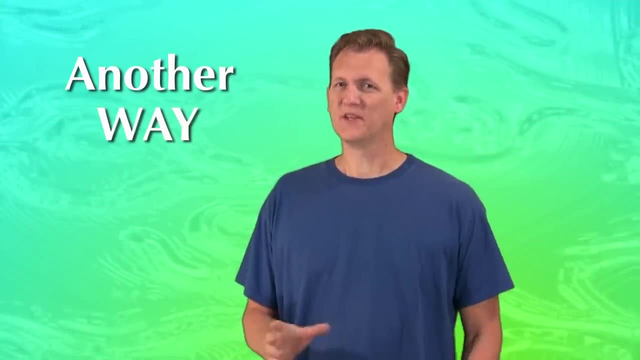 because its new top number, 99, is bigger. Pretty simple, huh. Okay, cross-multiplying is pretty cool, but there's another way to compare fractions that you need to know about, But this one's only really good if you can use a calculator. 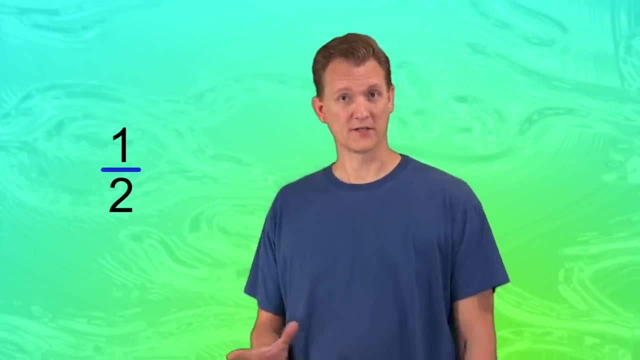 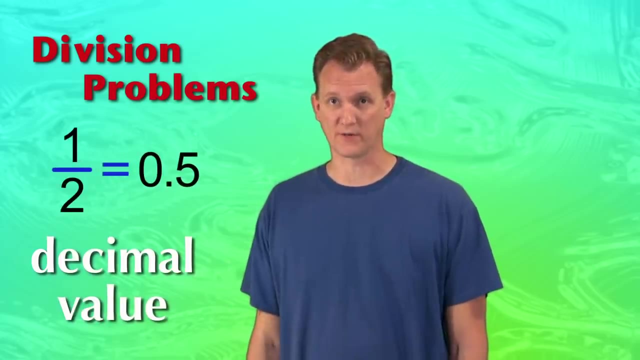 Remember, the reason that fractions are tricky to compare is because they're really division problems. But if we want to, we can just do the division and get the answer, which is the decimal value of the fraction. So if you have two fractions to compare, you can just do the division, preferably using 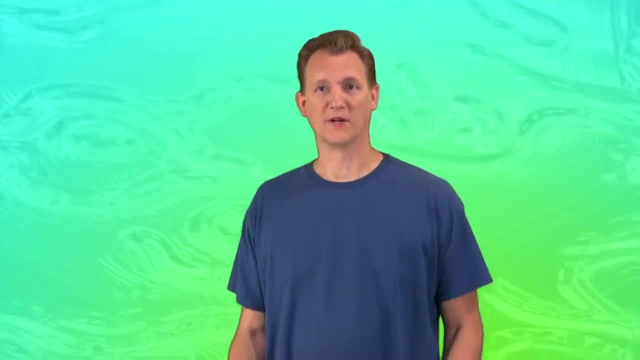 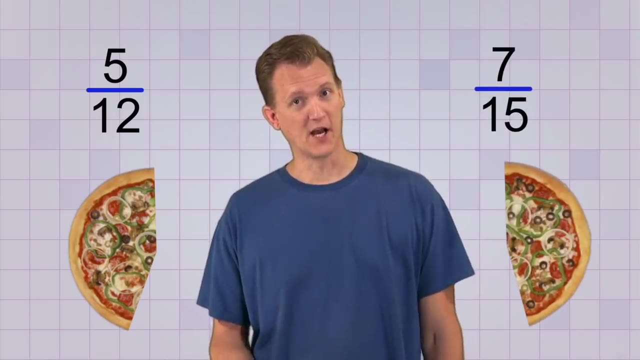 a calculator and then compare the decimal values. For example, Let's say I offered to give you either 5 twelfths of a pizza or 7 fifteenths of a pizza. Now you happen to be really hungry, so you want to choose the biggest amount. 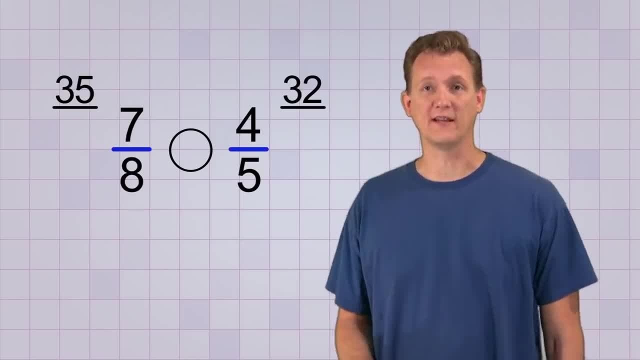 Aha, Now it's easy to see that the fraction 7 over 8 is greater than the fraction 4 over 5, because its new top number 35, is greater than the other new top number 32.. Let's do one more comparison by cross-multiplying. 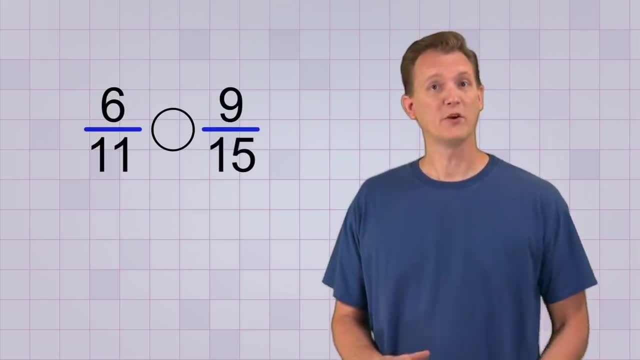 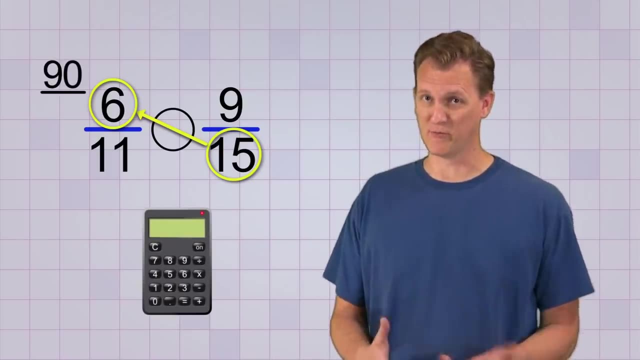 Let's compare 6 over 11 to 9 over 15.. First we'll multiply 15 by 6 to get the new top number of the first side, which is 90. You can always use a calculator to do the multiplications if you need to. 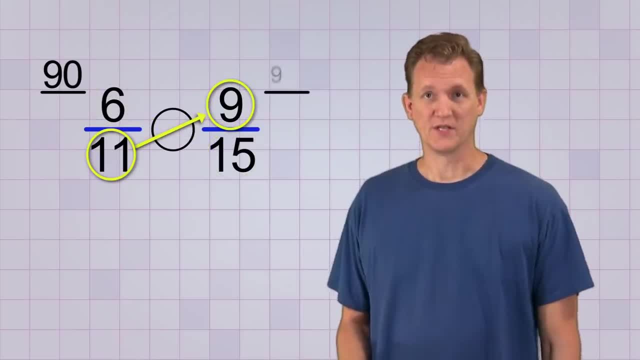 Next we multiply 11 by 9 to get the second new top number, which is 99.. So that tells us that the second fraction, 9 over 15, is greater than the first fraction because its new top number, 99, is bigger. 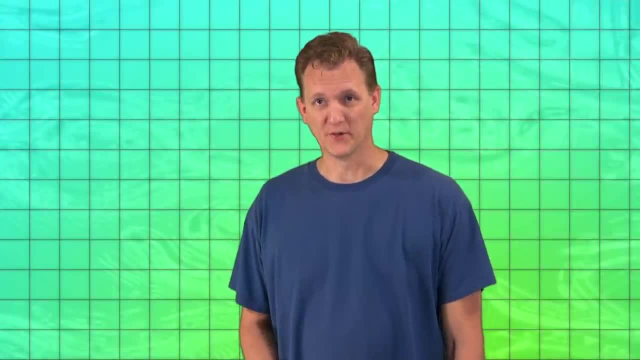 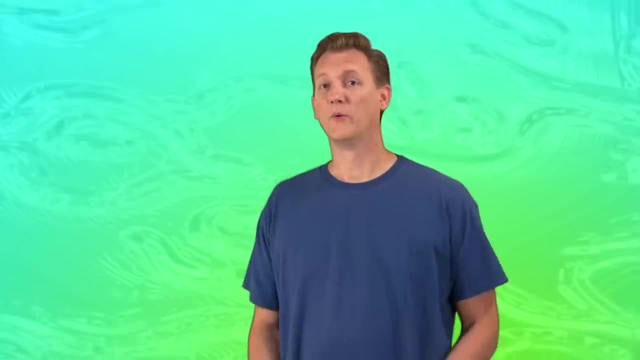 Pretty simple, huh? Okay, cross-multiplying is pretty cool, but there's another way to compare fractions that you need to know about, But this one's only really good if you can use a calculator. Remember, the reason that fractions are tricky to compare is because they're really division. 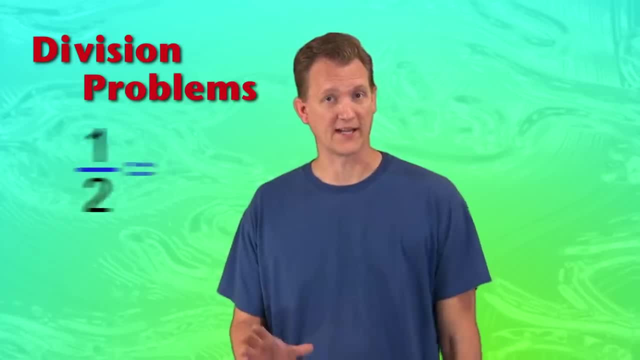 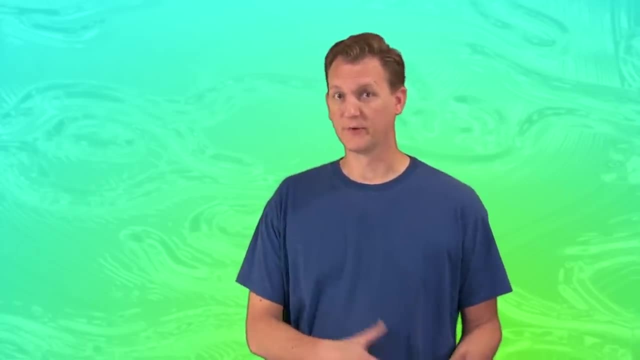 problems. But if we want to, we can just do the division and get the answer, which is the decimal value of the fraction. So if you have two fractions to compare, you can just do the division, preferably using a calculator, and then compare the decimal values. 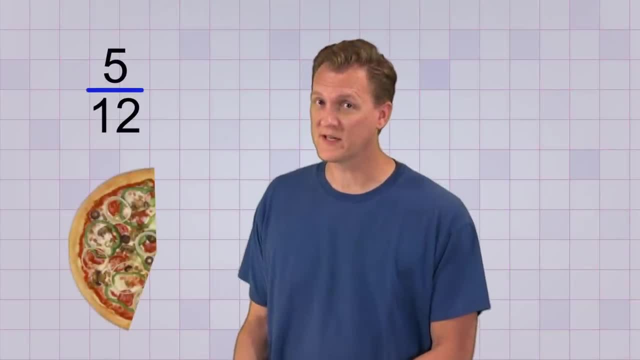 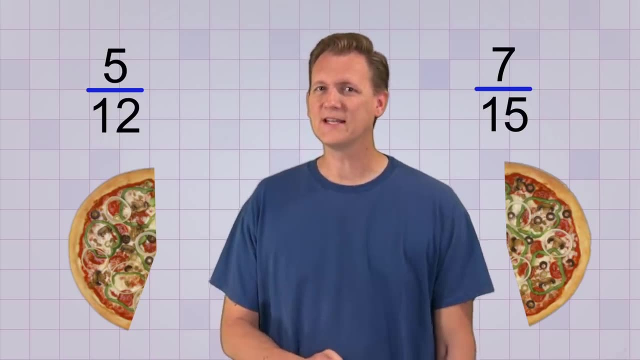 For example, Let's say I offered to give you either 5 twelfths of a pizza or 7 fifteenths of a pizza. Now you happen to be really hungry, so you want to choose the biggest amount. But it's not very easy to tell just by looking which is bigger: 5 twelfths or 7 fifteenths. 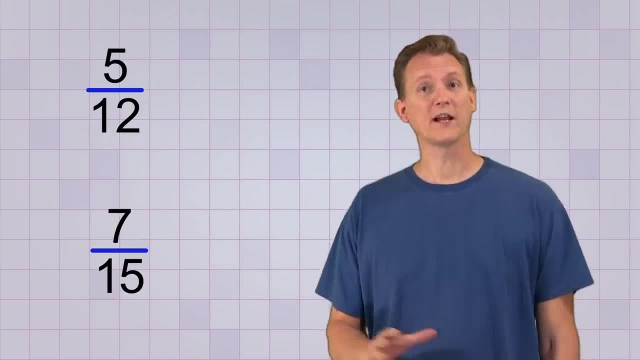 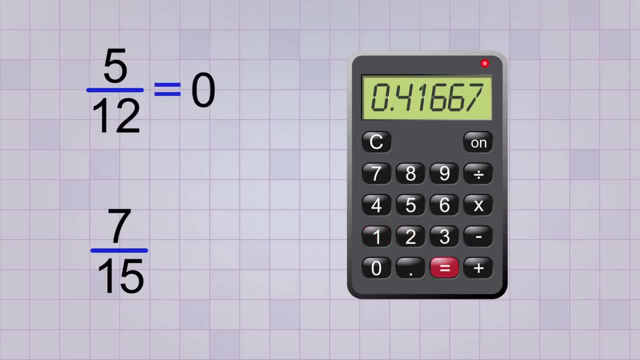 This is where decimal values can really help you out. If you convert the fractions to decimals by doing division, it will make it much easier to see which one's bigger. 5 divided by 12 is about 0.42, and 7 divided by 15 is about 0.47.. 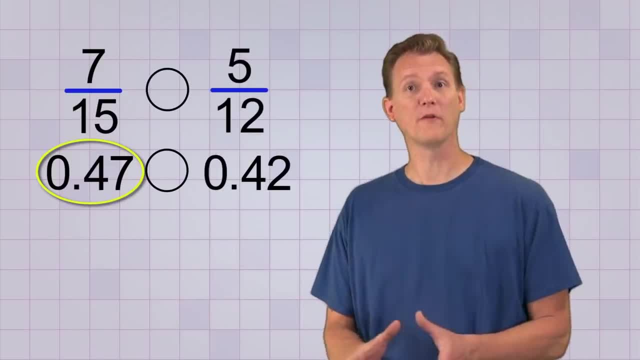 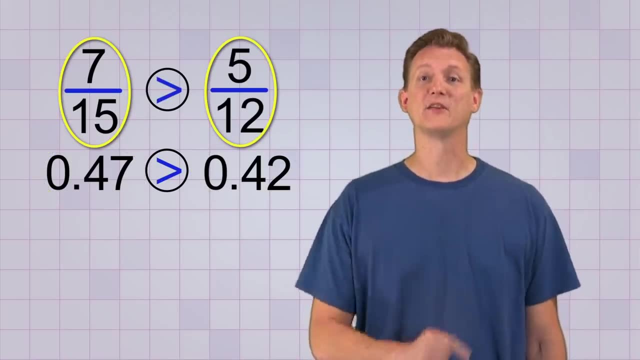 Yup, that makes comparing them MUCH easier. Since 0.47 is greater than 0.42,, it means that 7 fifteenths is greater than 5 twelfths, and that means that you'd rather have 7 fifteenths of the pizza. 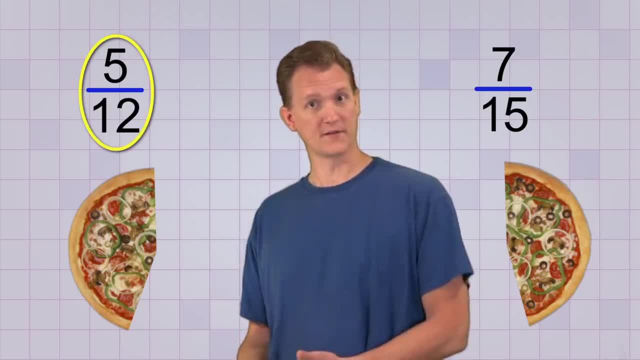 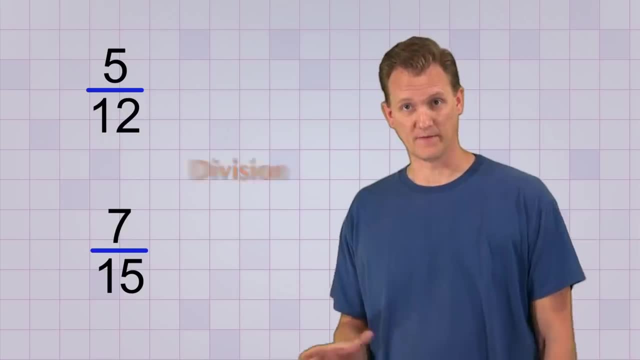 But it's not very easy to tell just by looking which is bigger: 5 twelfths or 7 fifteenths. This is where decimal values can really help you out. If you convert the fractions to decimals by doing division, it will make it much easier.